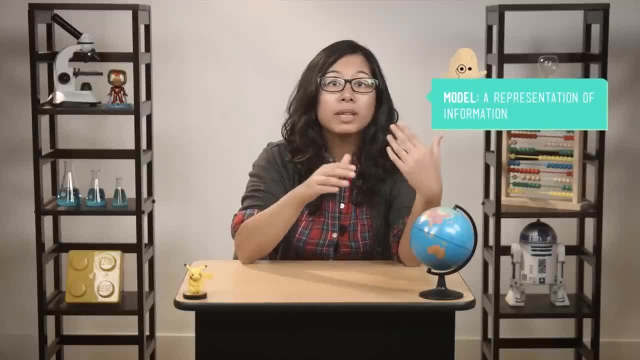 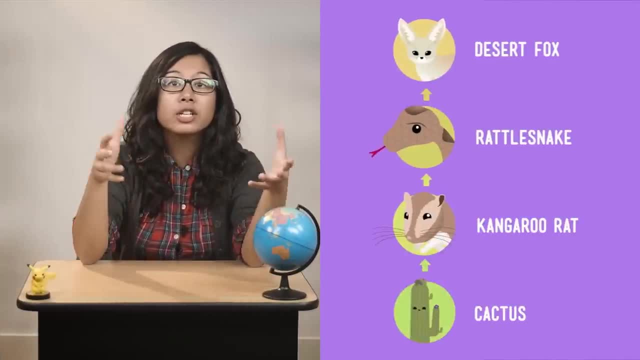 We can use a handy-dandy food chain model to see how energy flows between living things in this ecosystem. It would probably look something like this. The cactus makes energy by photosynthesis, and the energy goes from the cactus to the rat, then to the snake, and then to the fox. Now, although the cactus has adaptations that help it store and save water, it still needs rain. If it doesn't get enough in a drier climate, it's not going to have anything to store, and it's not going to be able to survive. And you know what happens when we take out the bottom of the food chain? It's like taking the wrong block in Jenga. We throw the rest of the ecosystem off balance. But that's not the only problem. Less rain and hotter temperatures mean less water to drink for all of the animals. And although they have adaptations too, like scales to help them retain water, that won't be enough to let them fit into a much hotter and drier climate. 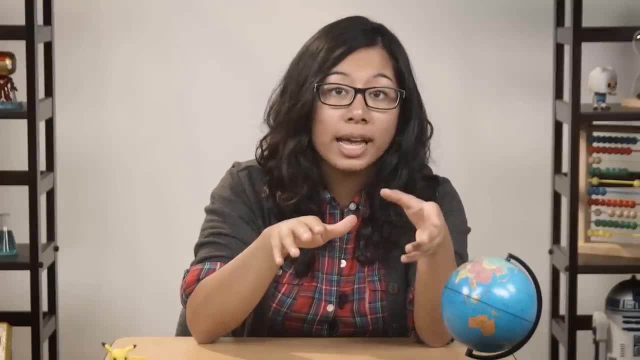 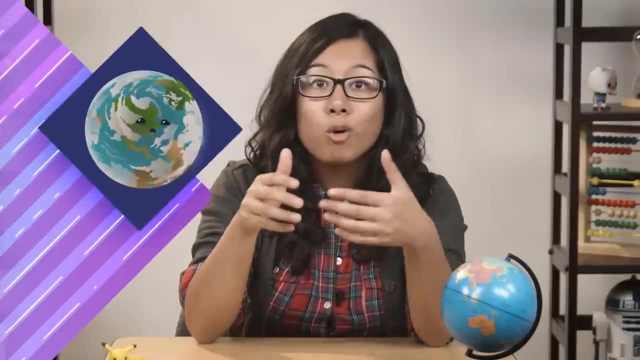 And globally, the climate is changing. Scientists who study climate change think that it's caused in part by changes to the Earth's atmosphere. An increase in gases, like carbon dioxide, is trapping more heat close to the Earth, acting like a blanket and making the Earth warmer. 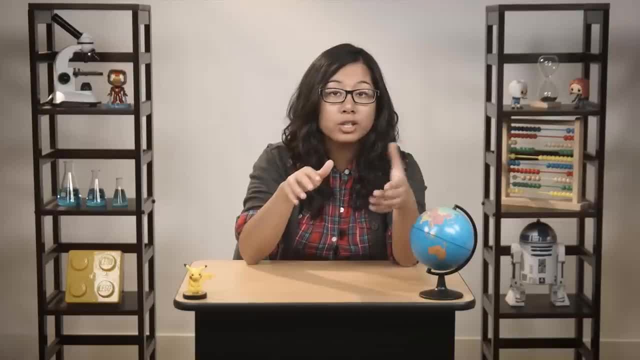 But scientists are hard at work trying to find solutions to climate change. For example, they're looking at ways to keep too much carbon dioxide from entering the atmosphere. 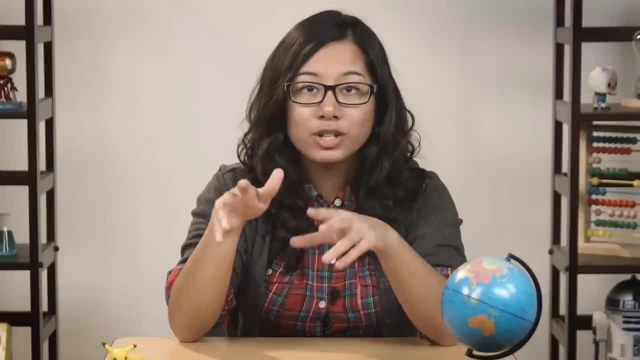 So, all living things that make up the Earth's biosphere have adaptations, characteristics that help them fit into their environment. Long-term changes in the Earth's weather patterns, called climate change, may have effects on the living things that make up ecosystems. 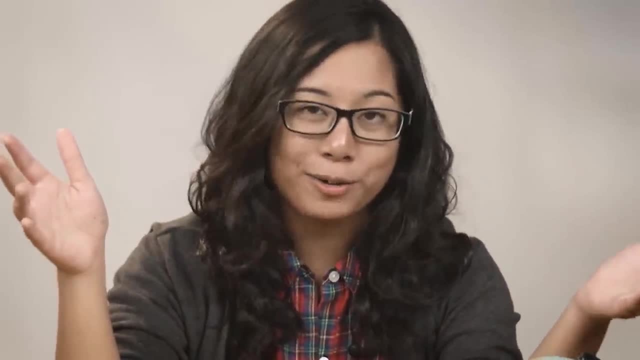 Now, if only I could change that! That joke I told at the beginning of this video. 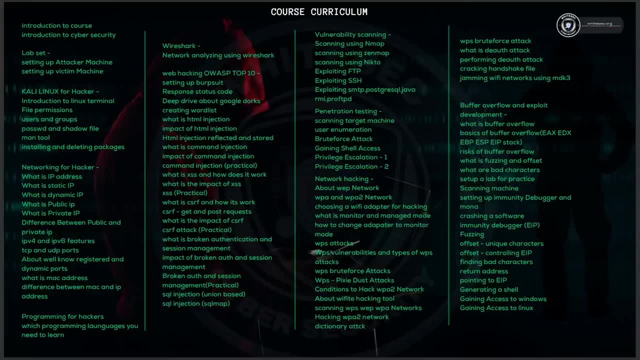 hello everyone, hope you are fine. in this training. you will learn ethical hacking right. so let me tell you, just try to watch this training in 1.5x because due to my slang, maybe sometimes i might be slow. okay, so the thing is, just try to watch it in 1.5x. and the second thing is, first of all, 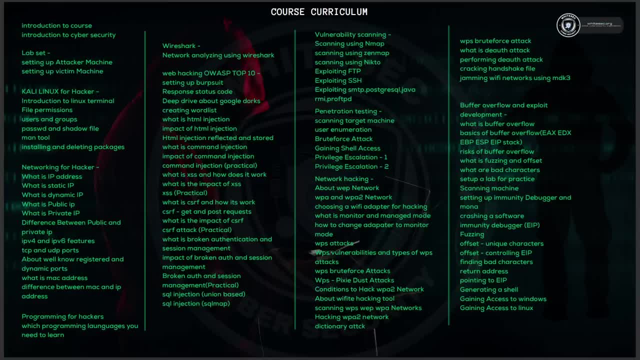 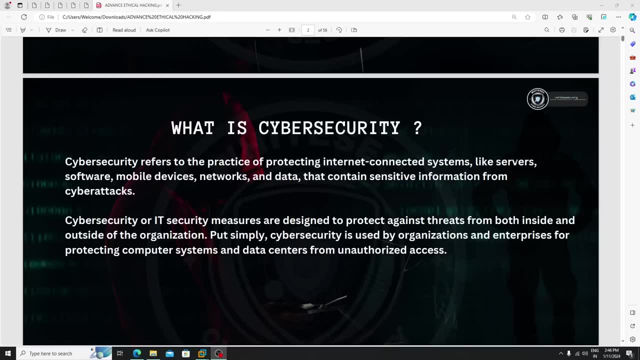 just try to watch the complete training, then practice it. okay, what is cyber security? cyber security refers to the practice of protecting internet connected systems like servers, software, mobile devices, networks and data that contain sensitive information from cyber attacks. the simple thing is you can also say it as a: the device which is connected with internet. 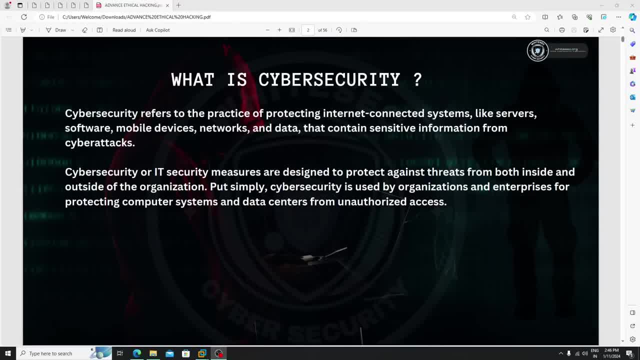 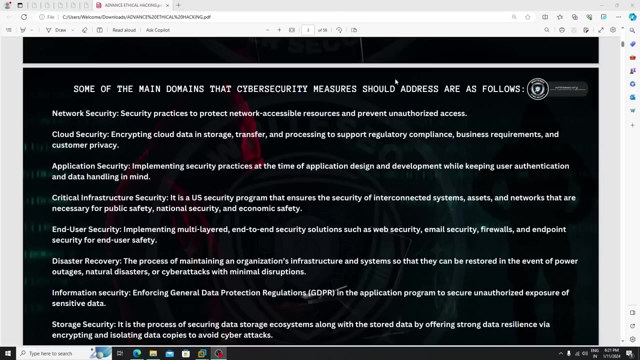 right. cyber security or it security measures are designed to protect against threat from both inside and outside of the organization. put simple, cyber security is used by organizations and enterprises for protecting computer systems and data center centers from unauthorized assets. some of the main domains that cyber security measures should: